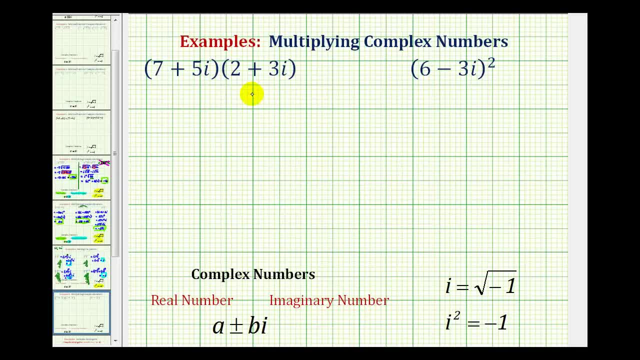 We want to multiply the given complex numbers. To do this, we'll multiply them algebraically, like we normally would when multiplying binomials. But then we need to make sure their product is in the form of a complex number or in the form a plus or minus bi. 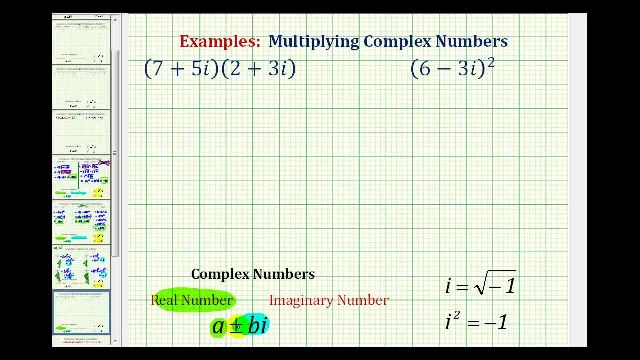 where a is a real number and plus or minus bi is an imaginary number, with i equal to the square root of negative one. So to find the product of seven plus five i and two plus three i, just as when multiplying binomials. 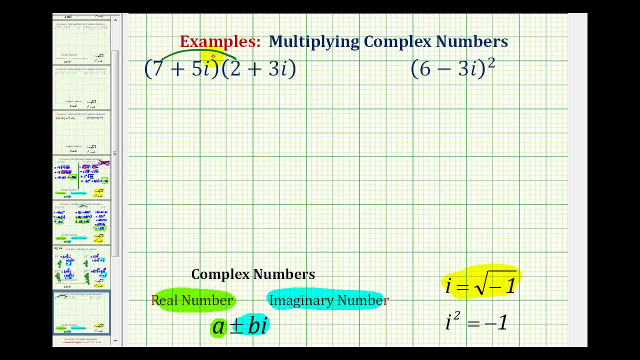 we'll have four products. We'll have one, two, three, four. So seven times two is equal to 14.. Seven times three i is equal to 21, i so plus 21 i. Then we have five i times two. 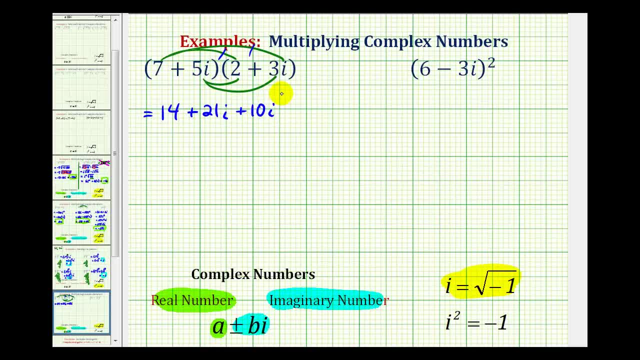 that's going to be plus 10 i. And then we have five i times three i, that'll be plus 15 i squared. Now we need to simplify this. Notice how the two middle terms are imaginary numbers, so we can add these two like we add, like terms. 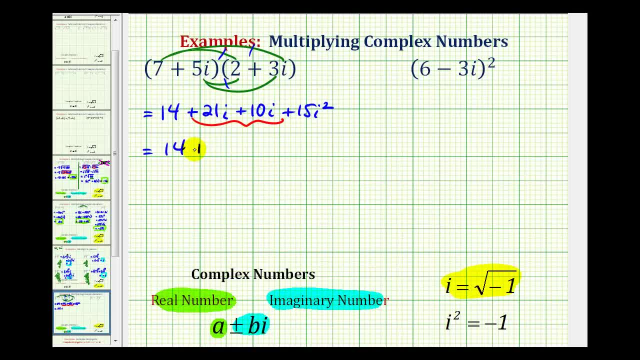 So we'd have 14, so it'd be plus 31, i plus 15, i squared, But we're still not done because, remember, a complex number must fit this form, so we need to simplify this. i squared, And since i squared is equal to negative one, 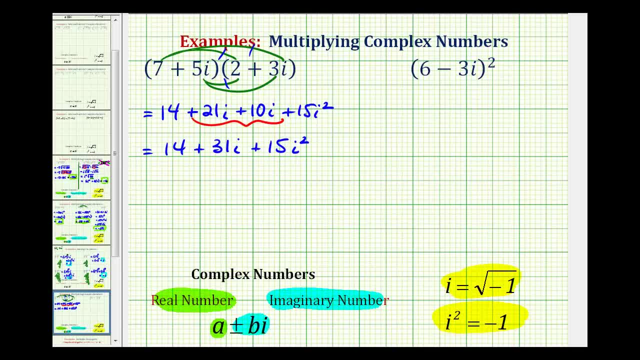 we can replace i squared with negative one. So we'd have 14 plus 31, i plus 15 times negative one. Well, 15 times negative one is negative 15.. And now we can add negative 15 and 14, which would be negative one. 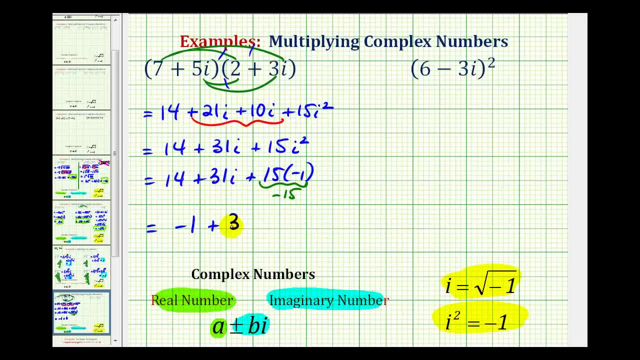 so our final product will be negative one. So that'll be negative one plus 31 i. When we give our final complex number, we should put the real part first and the imaginary part second. Next we have six minus three i squared. 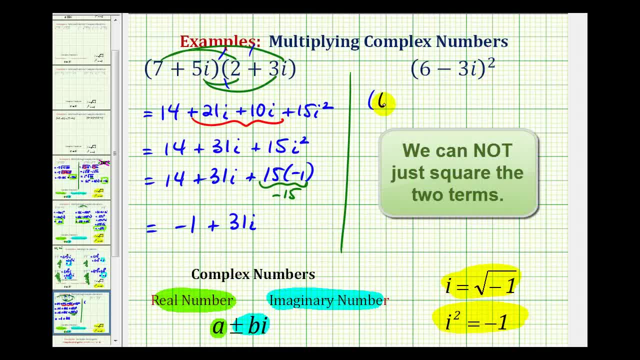 and there are no shortcuts here. We're going to have six minus three. i times six minus three i. And again we're going to have four products: One, two, three and four. So six times six is 31 i squared. 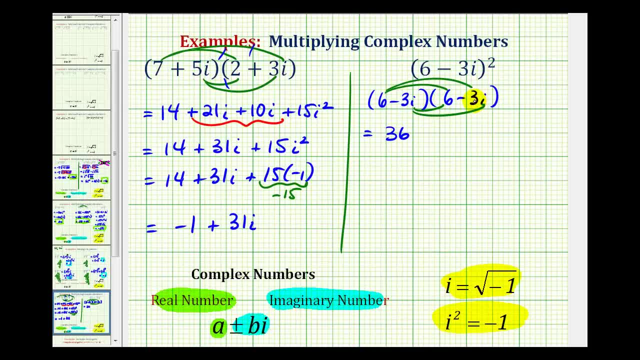 Six times six is 36.. Six times negative three i is going to be negative 18 i, And negative three i times six is also negative 18 i. Then we have negative three i times negative three i. that's going to be positive nine i squared. 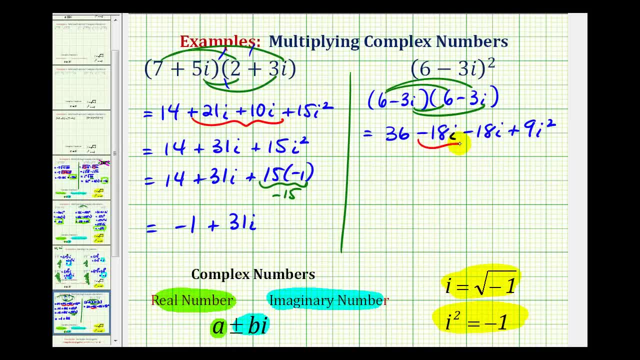 And now again, we need to simplify. The two middle terms are like terms or imaginary numbers which we can combine, And then we need to substitute negative one, for i squared So we'd have 36, this is going to be minus 36. i. 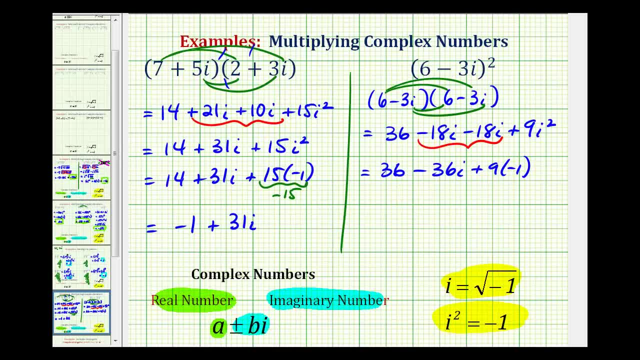 And then here we'll have plus nine times negative one. Well, nine times negative one is equal to negative nine. So now we can add 36 and negative nine, which would give us 27.. So our final product would be 27 minus 36. i. 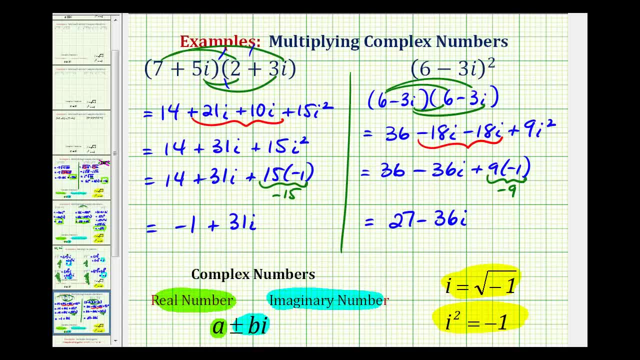 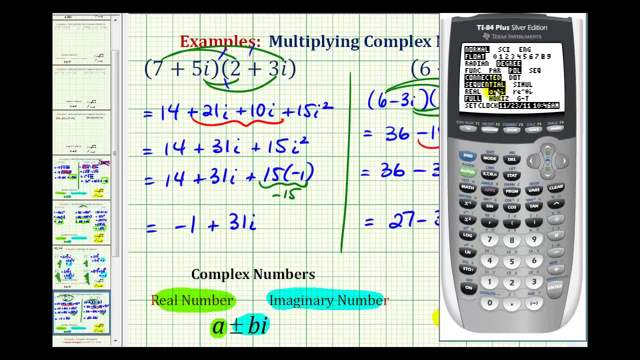 Let's go ahead and verify these. on the graphing calculator. We need to make sure we're in complex mode, so we'll press the mode key. Make sure we have a plus bi highlighted. Once we do, we can go back to the home screen. 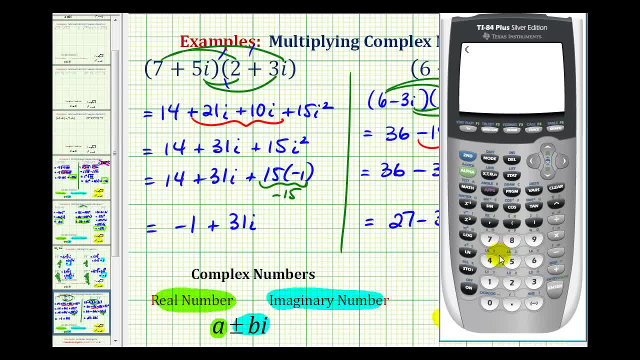 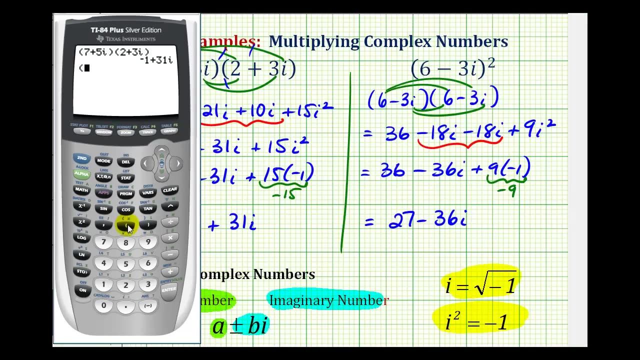 and just type in our products. So we first have seven plus five i- The i is second decimal point Times- two plus three i. This verifies our first product. And then we have six minus three i squared. We can press this button here for squared. 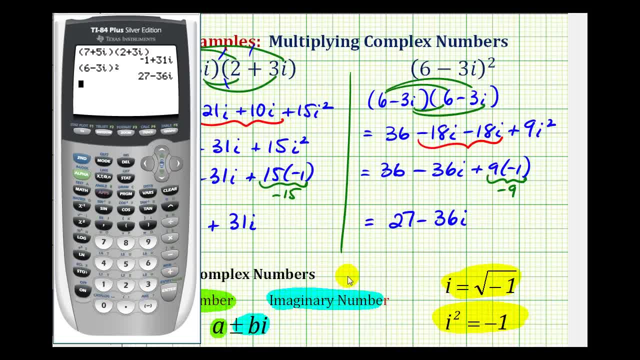 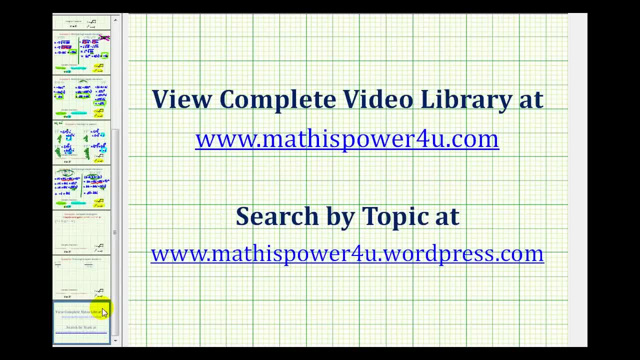 which verifies our second product as well. Okay, I hope you found this helpful. We'll see you in the next video.